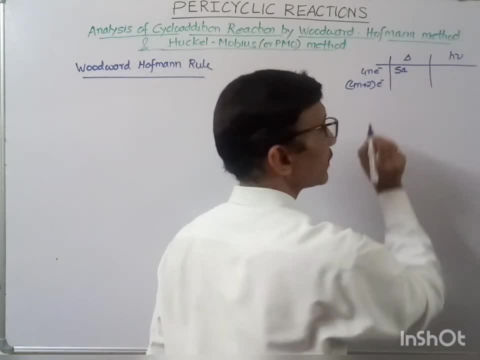 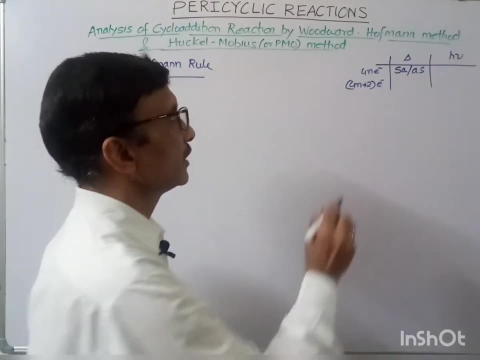 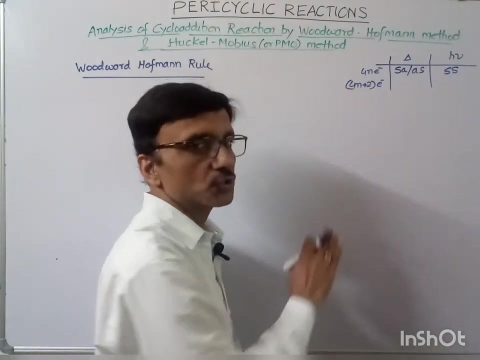 components interact in a suprafacial, intrafacial manner or intrafacial suprafacial manner. Whereas for photochemical condition, two component interact in a suprafacial suprafacial manner, Whereas for foreign plus two electron system, under thermal condition they interact in. 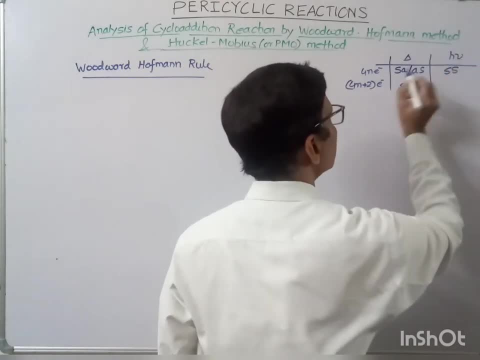 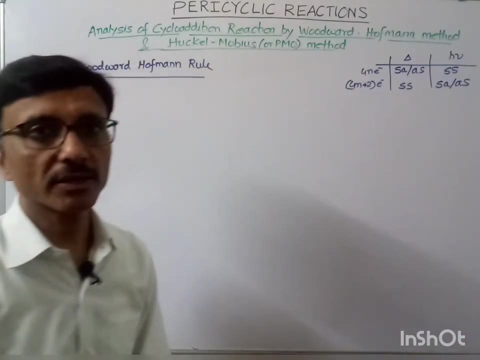 a suprafacial, suprafacial manner. Under photochemical condition, the two components interact in a suprafacial, intrafacial or intrafacial suprafacial manner. So this is the selection rule that we have to analyze by using this. 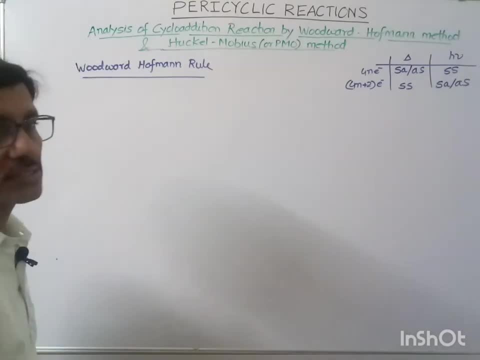 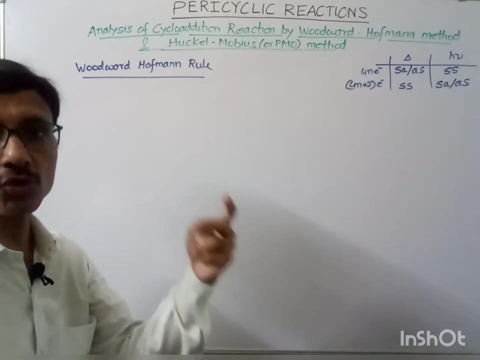 Woodward-Hoffmann rule. So what this rule says now, when either under thermal condition the reaction may be allowed or under photochemical condition reaction may be allowed. Now, out of these two conditions, no doubt superfacial or intrafacial, the reaction may be allowed. 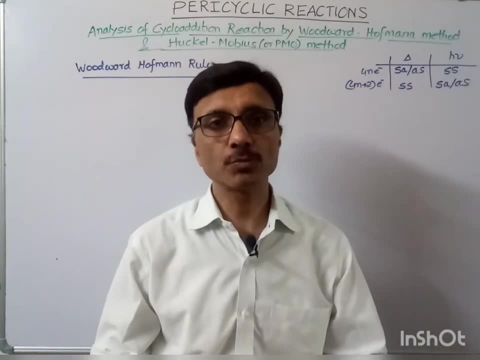 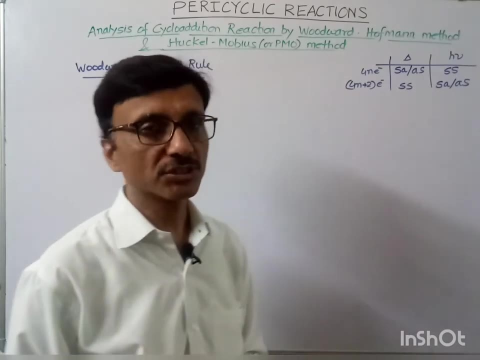 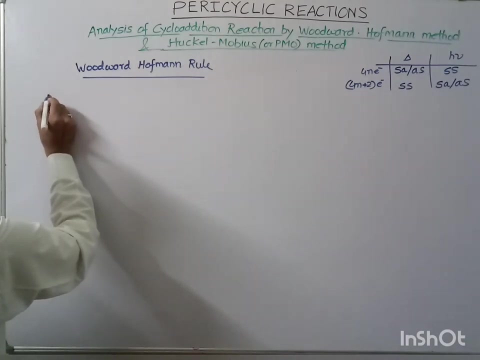 But without superficial suprafacial manner. the interaction in superficial suprafacial manner is favored over the suprafacial, intrafacial or intrafacial suprafacial manner. So if, according to this rule, the system is, we can write, the system is thermally. 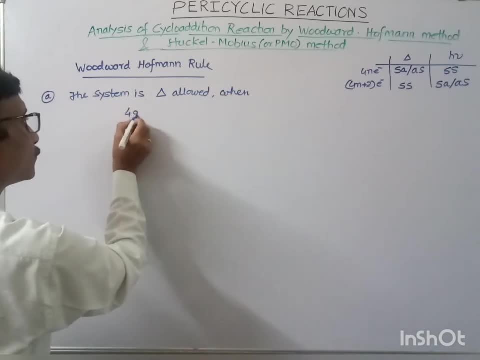 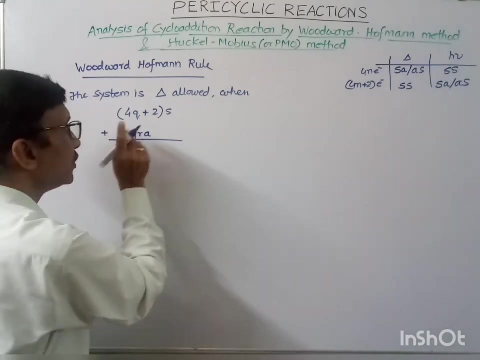 then the sum of two component, that is, 4Q plus 2S. this is one of the component and 4RA is the sum of these two component. If we add the sum of these, the value of these two component. okay. 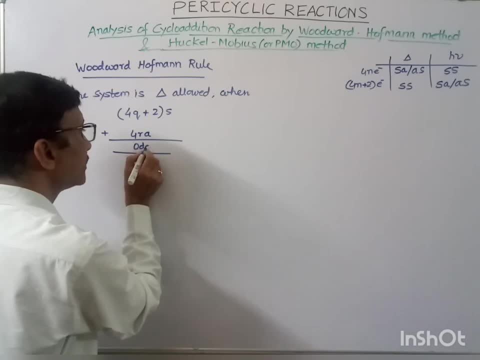 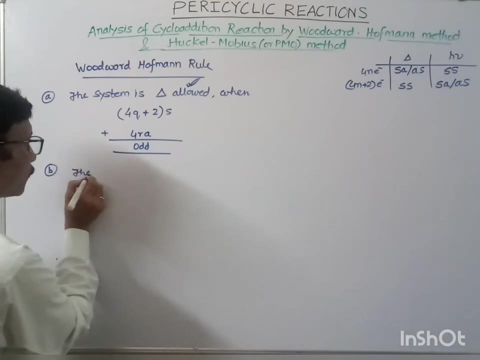 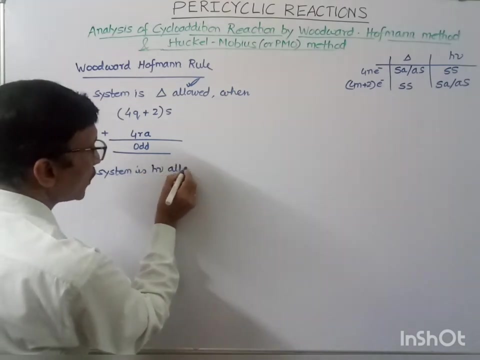 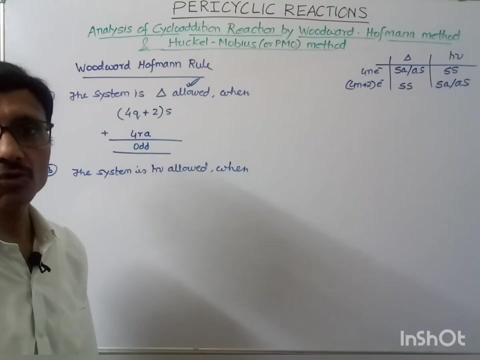 then if comes out to be odd, then it is thermally allowed. And when the system is photochemically allowed, under what condition? the system is photochemically allowed When the sum of these two component, they comes out to be even So, 4Q plus 2S. 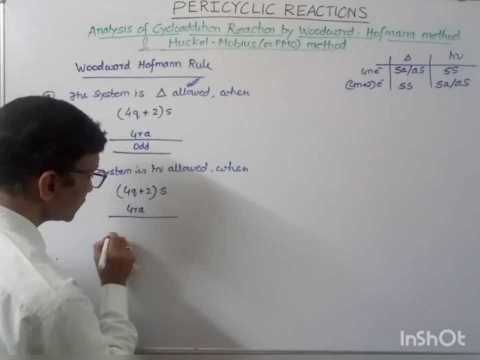 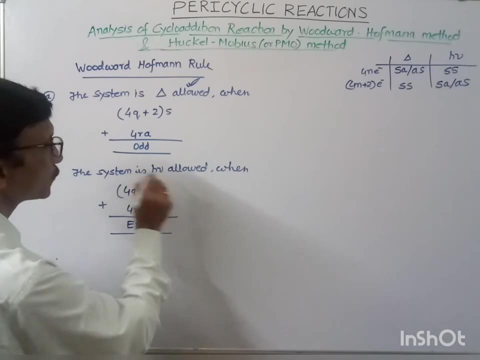 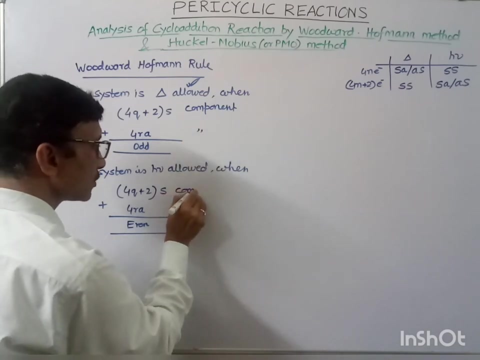 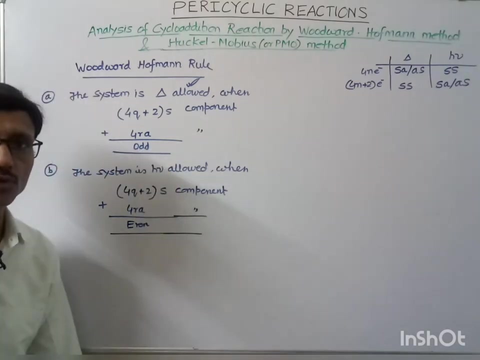 and 4 Ra. when this comes out to be the sum of these two component comes out to be, even then it is photo. or we can write this component, this component, sum of these two component comes out to be, even then it is: it is the coil. is photo chemically allowed? so we have two type. 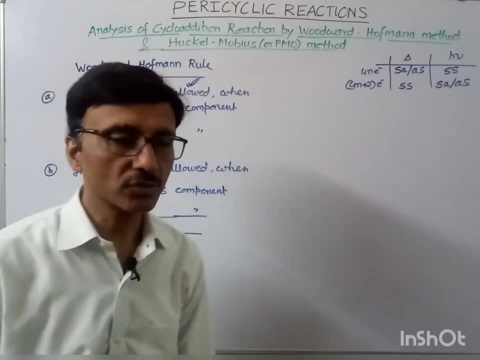 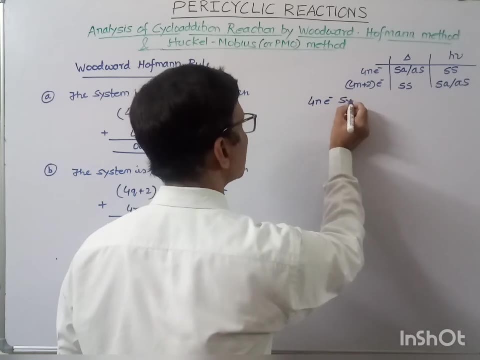 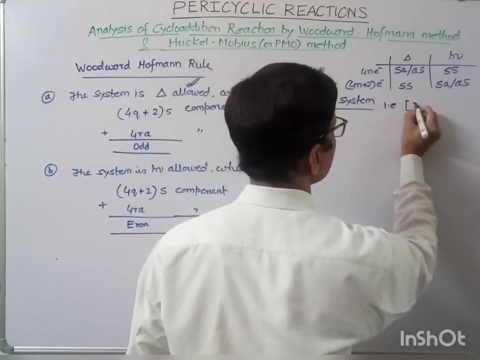 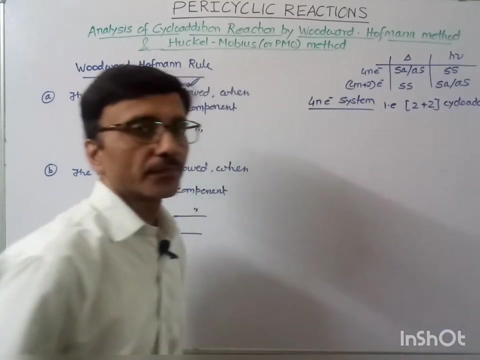 of system, either for an electronic system, for n plus 2 electrons system- I few stake the example of- for an electron system, for an electron system we add to place to addition, that is, the. that is 2 plus 2, second edition reaction, 2 plus 2, attention. okay, so you will see here then. 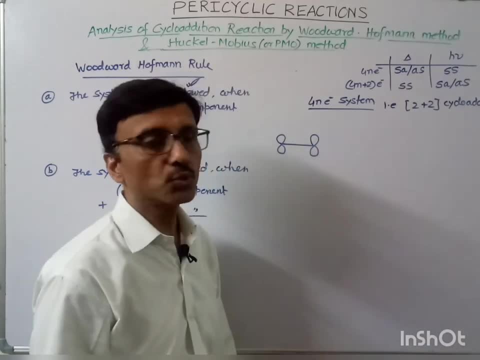 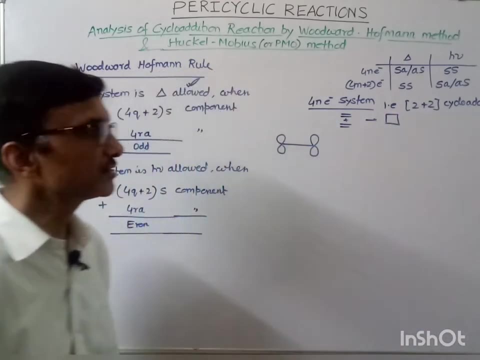 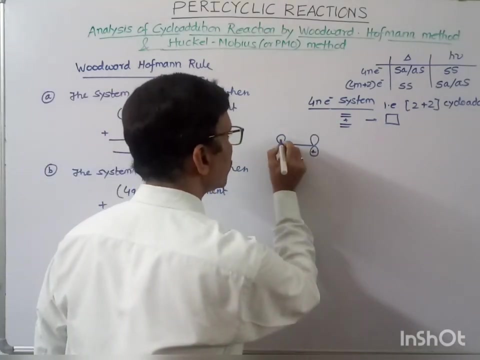 to plus 2. second reaction. Simplest example is the when two ethene and these two ethylene system, they react and it is giving this one. This is the simplest example. So the lobes of these two that will interact. So we should write, we should not take for. 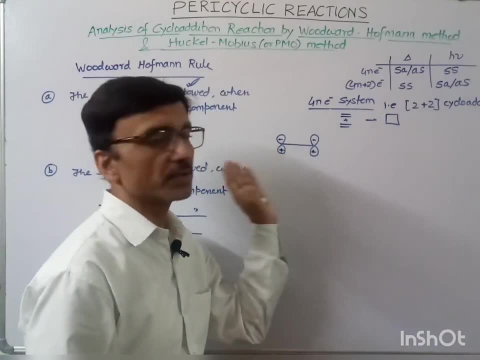 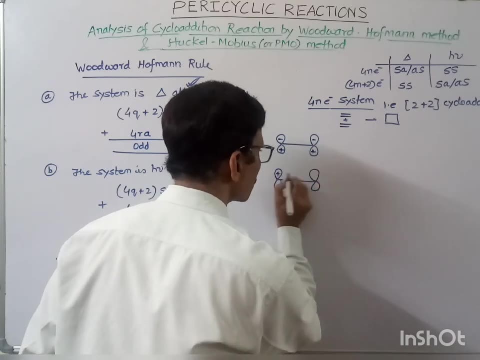 this one. for this rule we have to take simply plus, plus, plus, plus, all plus plus, like this first ethene system. second one: This should also be taken as plus plus. We should not take the homo or lomo like the FMO method. okay, We should not. 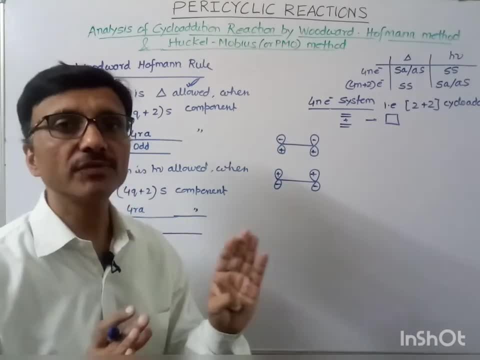 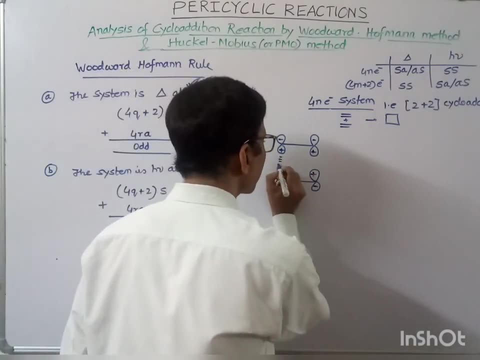 take the. we should not follow here the FMO method. We are not concerned with the homo or lomo, So simply we take the plus, plus, plus plus, and let's see one. Suppose they are interacting in this way On out superficial. superficial interaction is 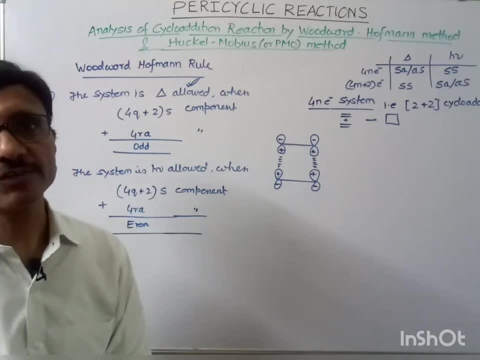 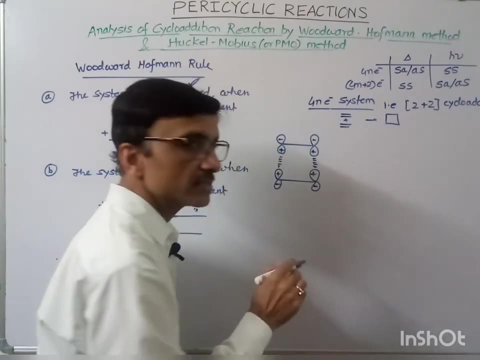 followed, It is favored. So when this superficial, superficial interaction is favored, So let us see. So what kind of this component? now it become V, Because they are adding in a S manner. So in my previous lecture I told you what 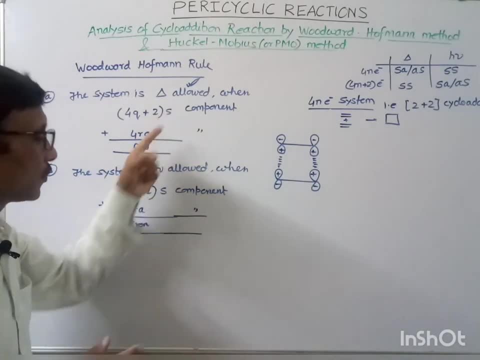 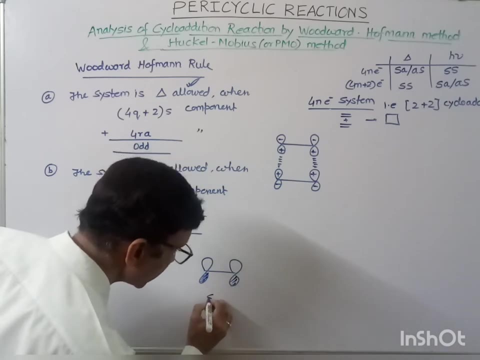 is the meaning of this S and A. I told you what is the meaning of S and A. So if anything which is which is interacting here, If same side lobe is interacting, then this is S component. If different side lobe is interacting, then this is A. 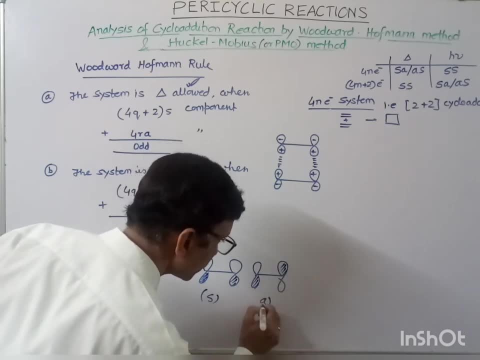 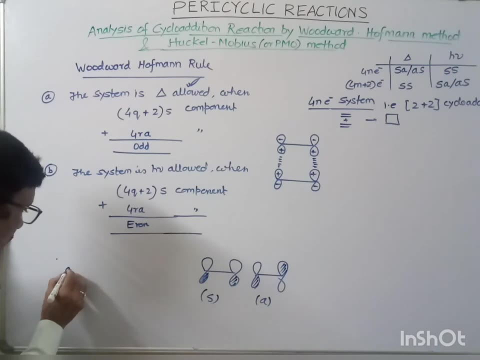 component. This is our A component. This is What about 4Q plus 2S and 4RA. So when suppose, if Q comes to be: If q is one zero, one, two, like this, Then such component is said to be to 4, Q plus 2 component. This is 4Q plus. 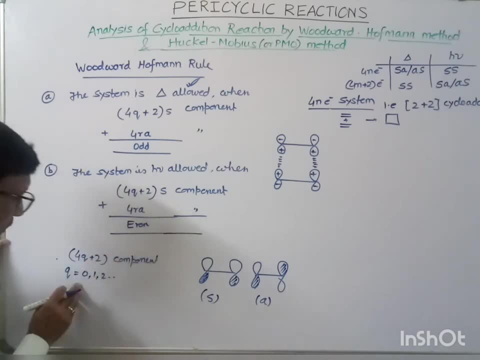 two component. When Q comes out to be 0, 1, 2 and when R comes out to be 1, 2, 3, like this, Then this is n is said to be 4R component. So two type of component you. 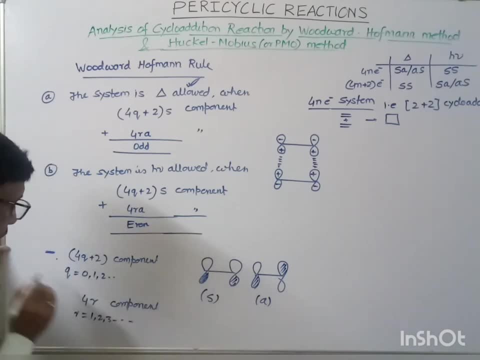 here. One is 4Q plus 2 component and another is 4R component. Now what about this? whether this is 4Q plus 2 or 4R? So, if you will see, if you put Q is equal, to suppose I am putting Q is equal. 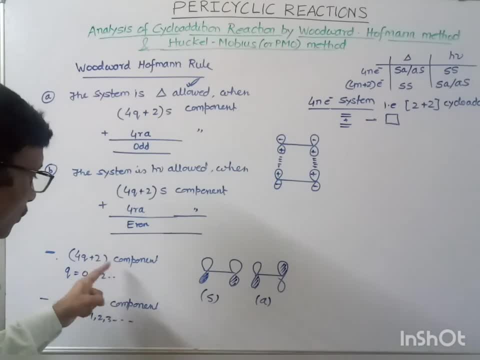 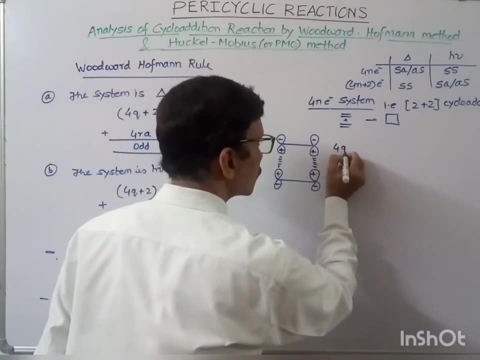 to 0, then we get 2 electron, 2 component. So this is 2 electron, 2 electron. that's why this is 4Q plus, this is 4Q plus 2.. Now 4Q plus 2, whether this is S or A, this is because same. 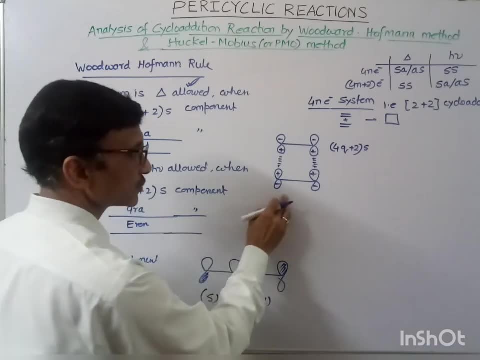 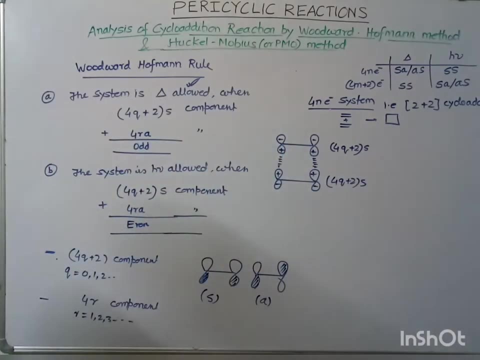 side lobe is interacting. this is S Same for this one, because same side lobe. this is also 4Q plus 2S. this is also S. Now we should see whether this is this is thermally allowed or photochemically. 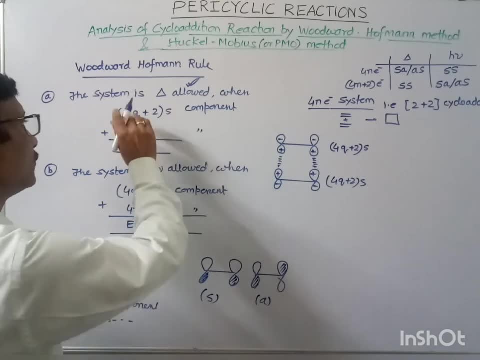 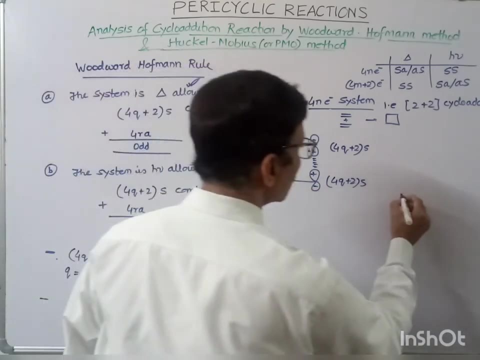 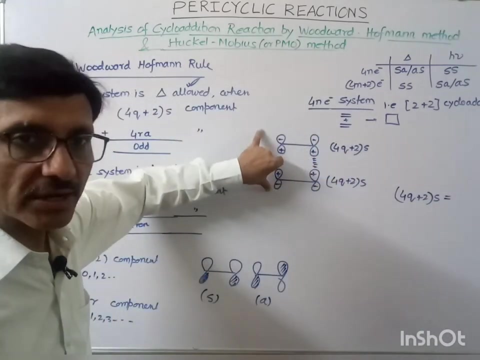 allowed, Whether this is thermally allowed, photochemically allowed. we should see the sum of these. Let us see the sum of these two components Now, in this case 4Q plus 2S. how many such components are there in this interaction? Two components, So in this interaction, two such. 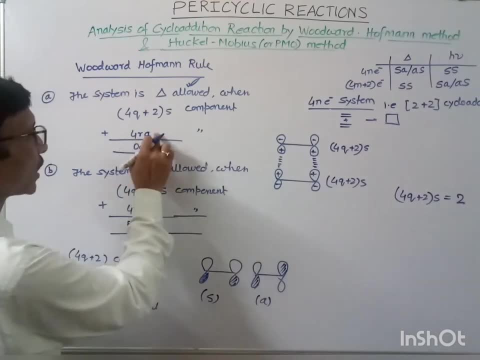 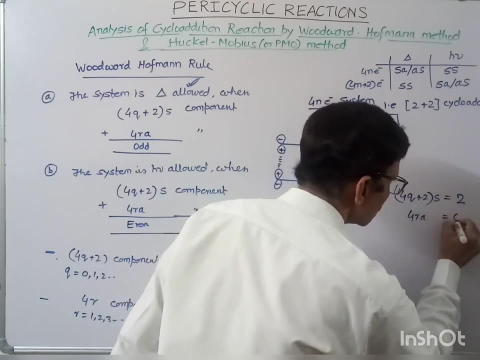 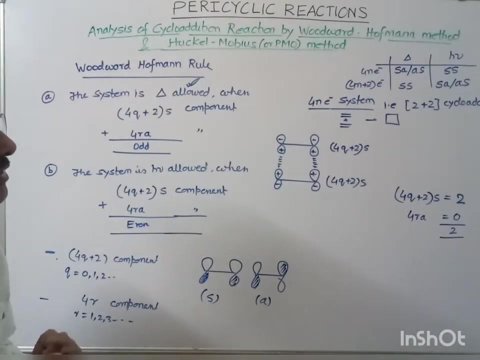 components are there Now 4RA? how many 4RA component is there? No 4RA component? So 4RA, this is equal to 0. So this comes out to be total 2.. So this is coming to be even. So if this is even, it means such interaction for 2 plus 2. 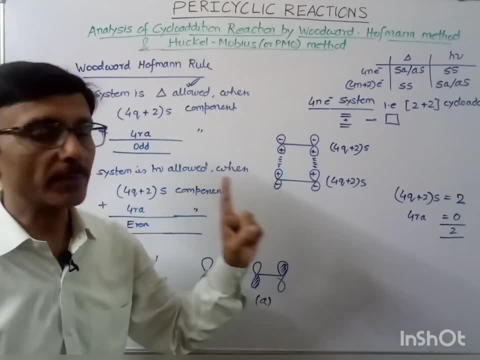 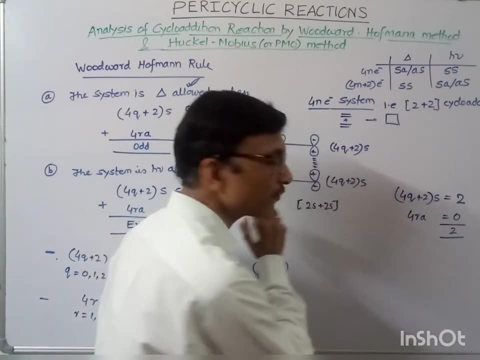 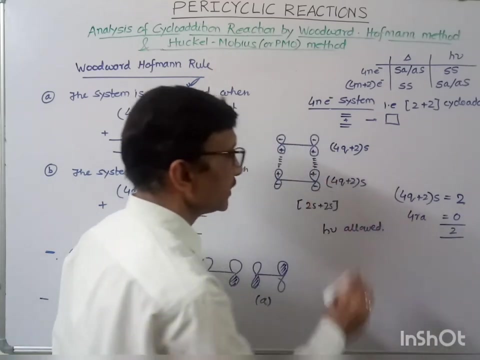 cycloaddition reaction. such interaction is allowed photochemically only. So this means: this is what kind of interaction this is. This is 2S plus 2S interaction, that is, superficial-superficial interaction. So that's why it is photochemically allowed. It is photochemically allowed, Okay Now. 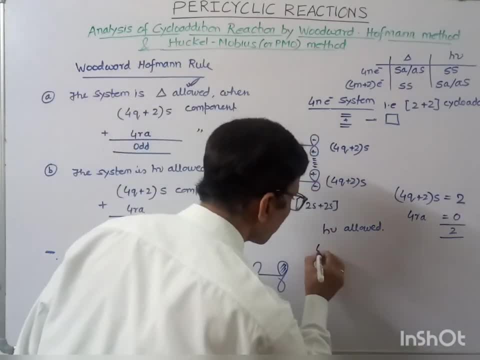 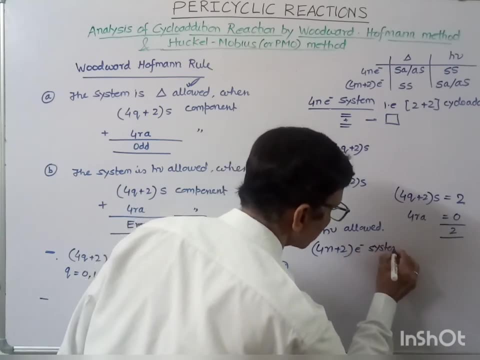 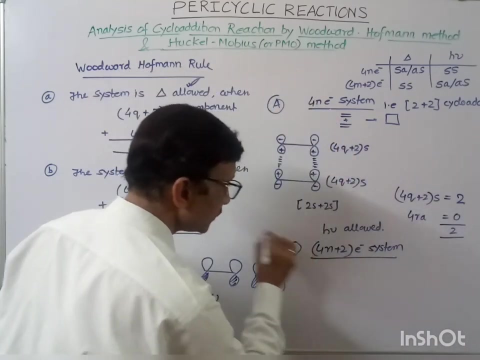 so now for 4N plus 2 electron systems. if you see, for 4N plus 2 electron systems, Let us check for this one. So this is case A or for N electron system. This is case D for 4 buy 2. 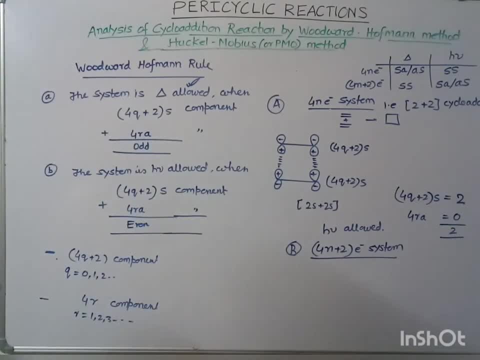 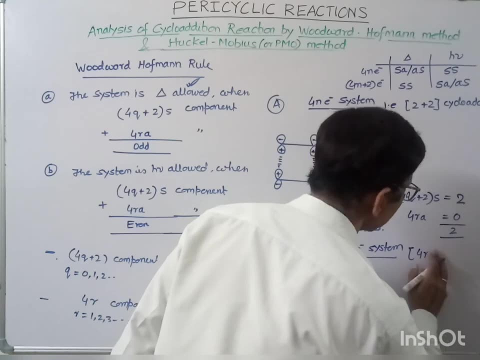 electron system. Now for this one that is 4.. That is, you can say this is 4N and that order is is: it is 4 plus 2 cycloaddition reaction. this should be 4 plus 2 cycloaddition. 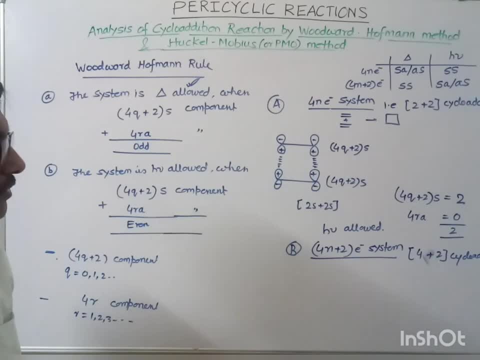 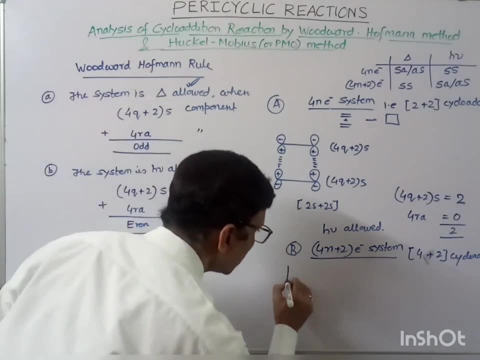 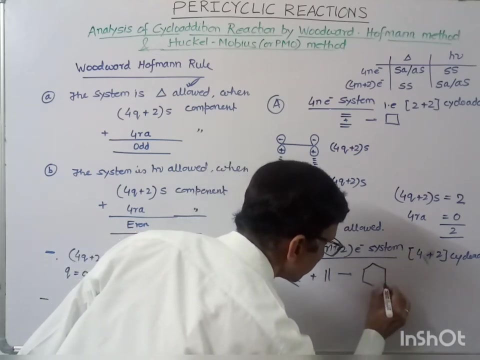 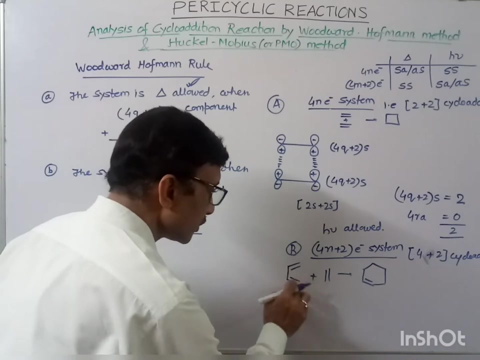 reaction: okay, this is 4, 4 plus 4n plus 2 cycloaddition: the 4 plus 2 cycloaddition reaction. the simplest example: when this butadiene, it will interact with the ethene and you get the cyclohexane. okay, now, so how you see? now we should draw the. 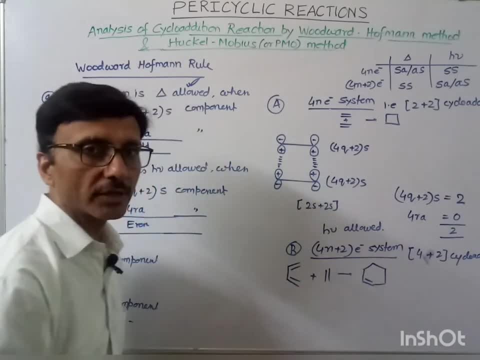 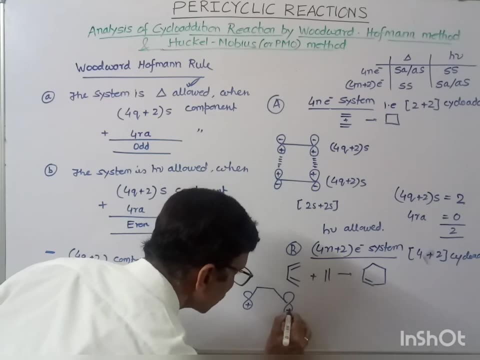 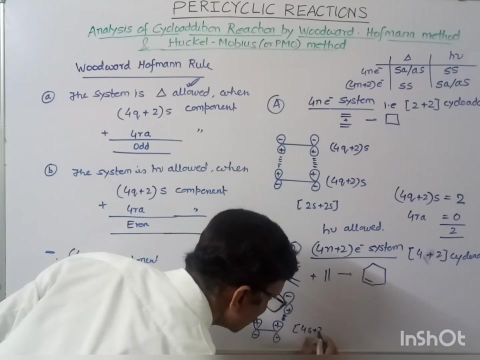 terminal loop for this one and terminal loop for ethene. terminal loop for this butadiene plus plus- we are only concerned with this one- and terminal loop for this ethene plus plus, minus, minus. now, when this superficial, superficial interaction is allowed, let us see. so here these are interacting in your, but kind of manners, 4s plus 2s manner. this 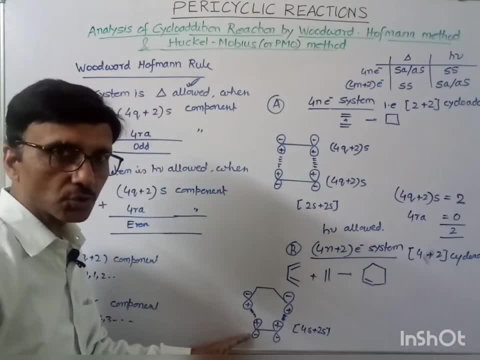 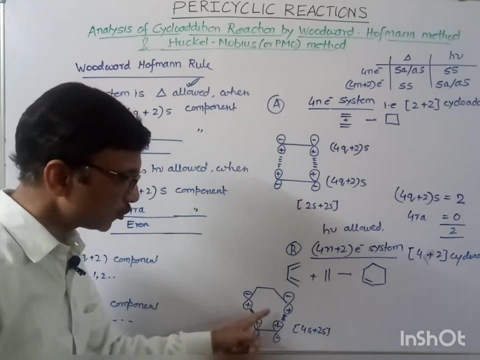 is. this component is 4s. this component is 2s. that's why I have written 4s plus 2s, because this is interacting in a superficial manner. same side lobe is interacting here also, same side lobe is interacting, that is, in superficial. 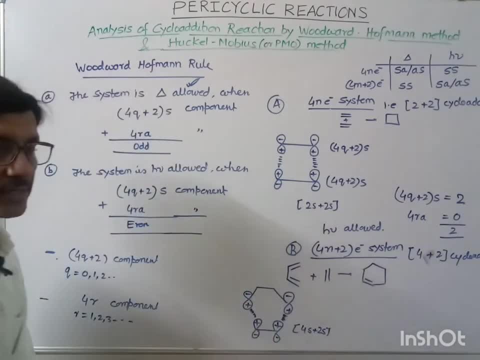 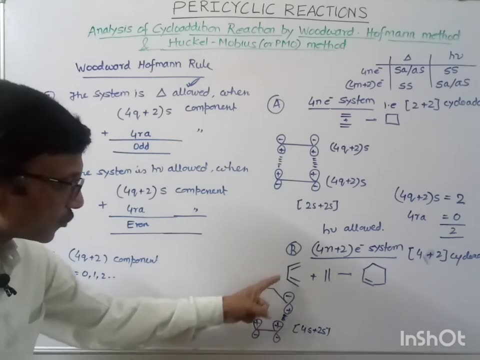 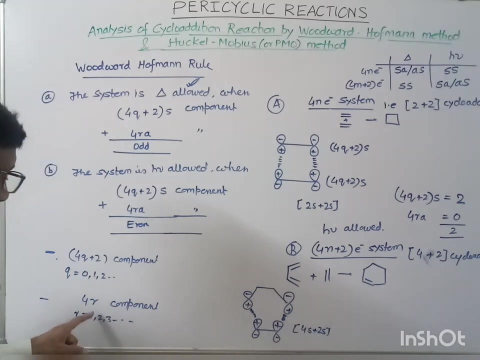 manner. that's what is true. 2s. Now, what kind of component this is? Either this one or this one. Now. so if this is how many electrons are present over here, 4 electrons are present. So if we put r is equal to 2, then we get. 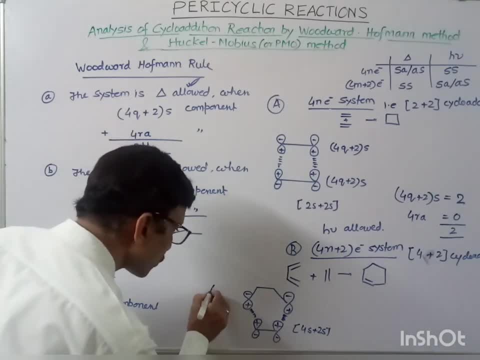 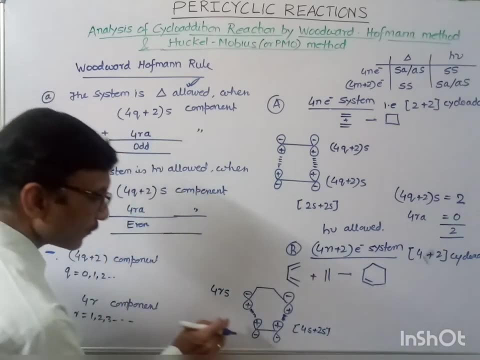 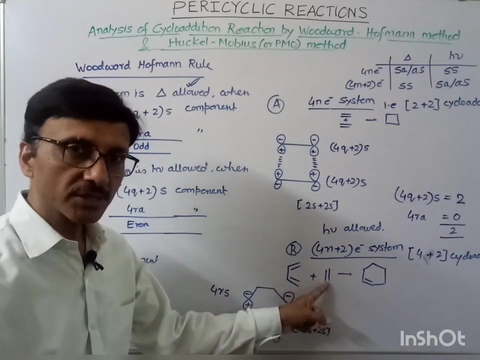 the 4r component. So this is 4r and as they are interacting in a superficial manner, that's what is 4rs component. What about this? What about this? How many electrons are present over here? The electron present is 2 electrons are present over here and this is interacting in a superficial. 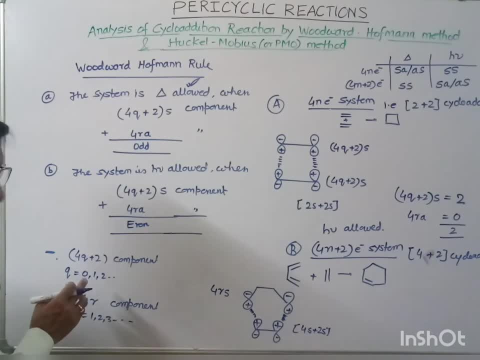 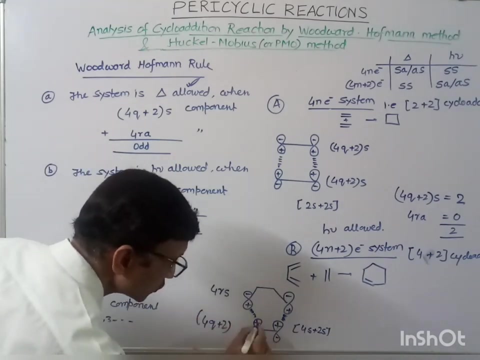 manner. So 2 electrons means 2 electrons. When the 2 electrons come When q is equal to 0.. When q is equal to 0, then it means this is 4q plus 2 and s This is 4q plus 2.. Why s? Because 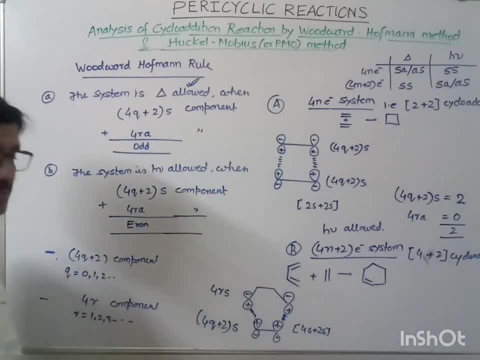 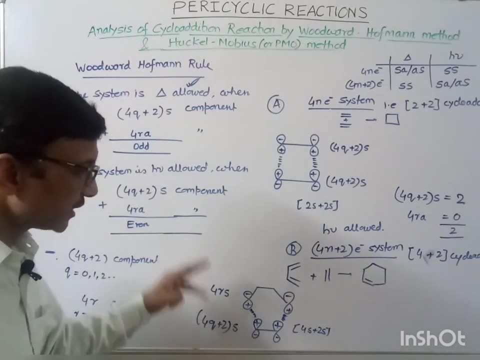 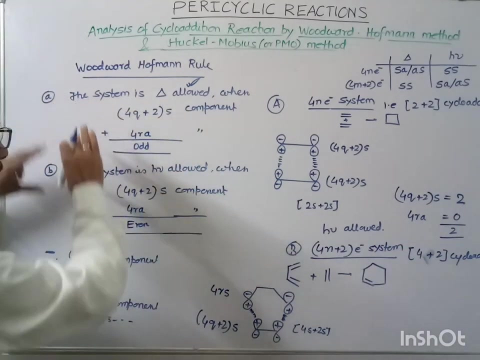 they are interacting in a superficial S Same side lobe is interacting. That's what is. 4q plus 2s. Okay Now. so let us see their sum. Let us see whether this is thermally allowed or this is photochemical error. For this we should follow this rule Now: 4q plus 2s. How many 4q plus 2s? 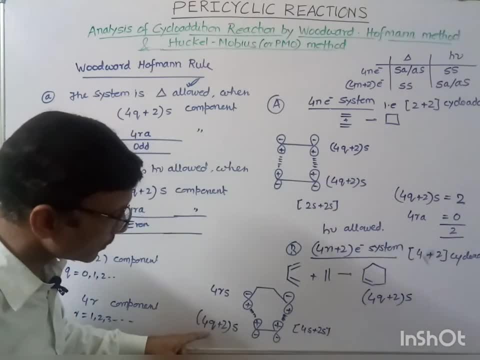 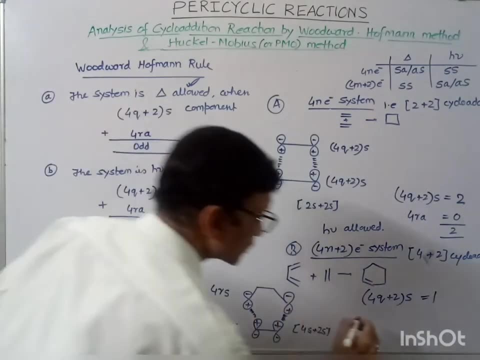 component are there? How many 4q plus 2s component is there? Only one 4q plus 2s component is there. How many 4ra component is there? 4ra component? So if you will see 4, there is no 4ra component. 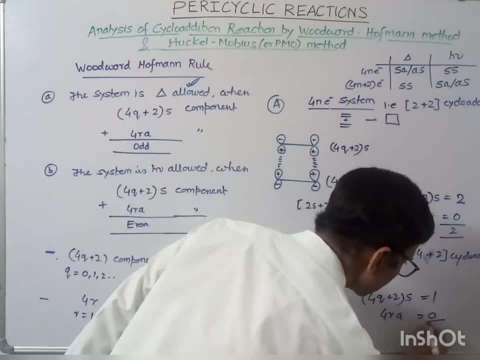 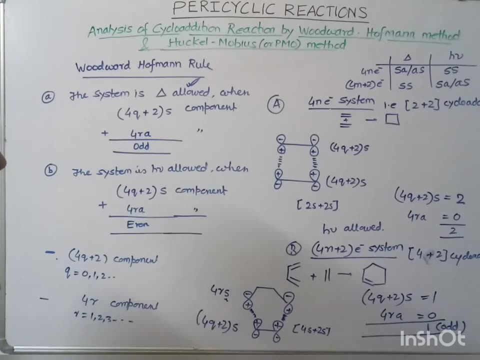 This is 4s component. So that's why 4ra component is 0 and is coming out to be 1 and this 1 is odd. So if 1 is odd, then it means it is coming odd, That is, this is thermally allowed. So for 4n: 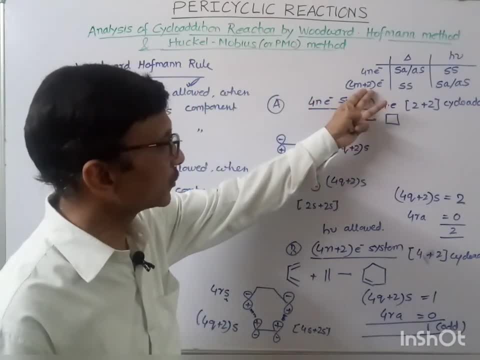 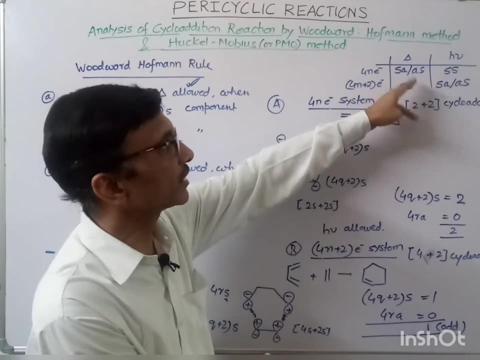 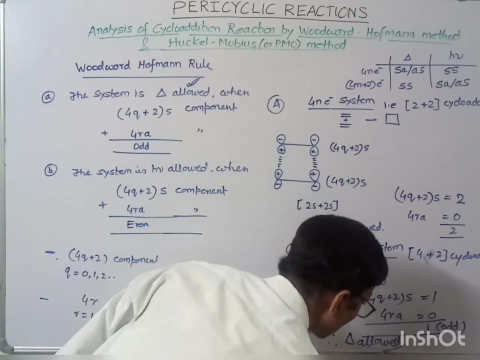 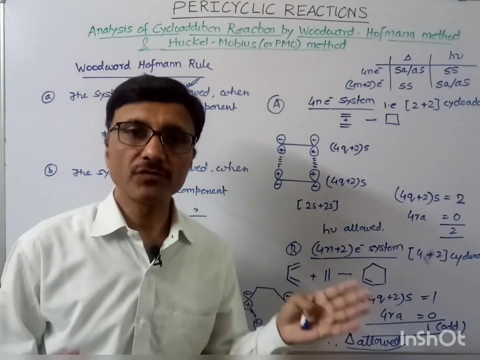 plus 2 electron system. If the orbitals are interacting in superficial, superficial manner, then they, only they- will interact under the thermal condition. So therefore it is thermally allowed. Okay, So this is about the Woodward-Hoffman rule, So you may also go to the Woodward-Hoffman. 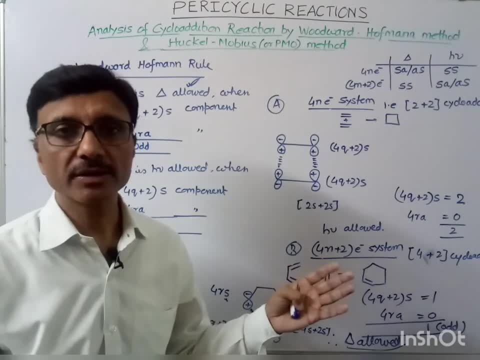 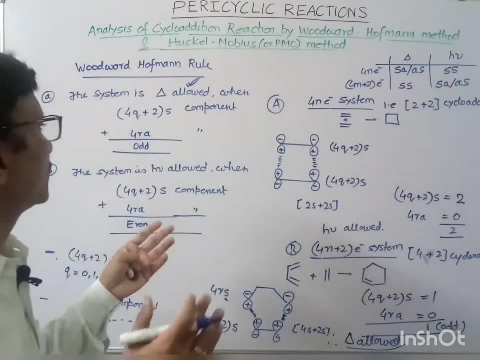 rule for the electrocyclic reaction and in a same manner, you may see the analysis of this rule in a same manner. So this is the analysis of this rule. So this is the analysis of this rule in a same manner. We can analyze, Only the rule was different for this. 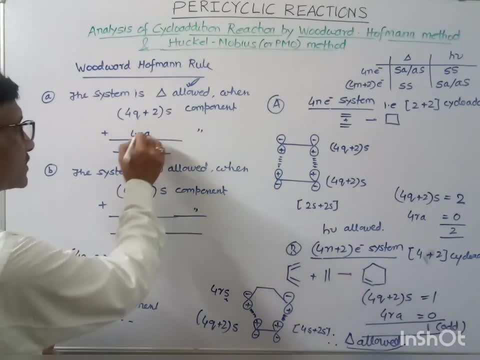 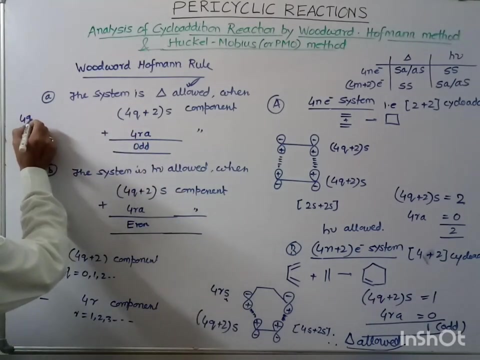 OK Here this rule tells that 4q plus 2s, and this is odd. So according to that one, in electrocyclic reaction what we read is 4q plus 2s. This, if it comes to be odd, then this is thermally allowed. And if 4q plus 2a and 4rs, if this comes out to be. 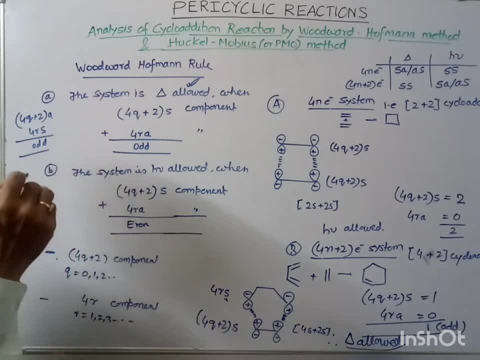 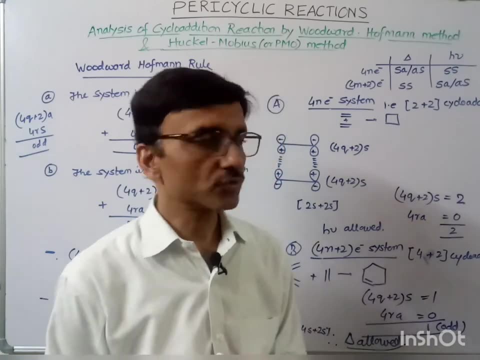 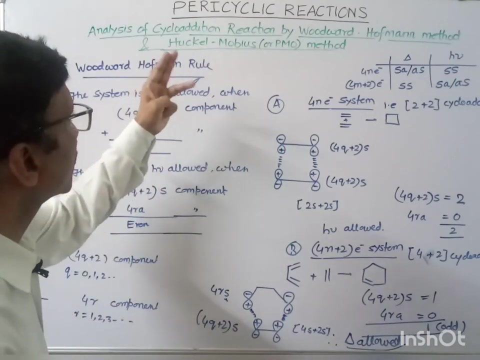 odd. if this comes out to be odd, then this was photochemically allowed, So slight change in rule was there in case of electrocyclic reaction. Now let us see the analysis of cycloaddition reaction by Huckel-Mobius method. 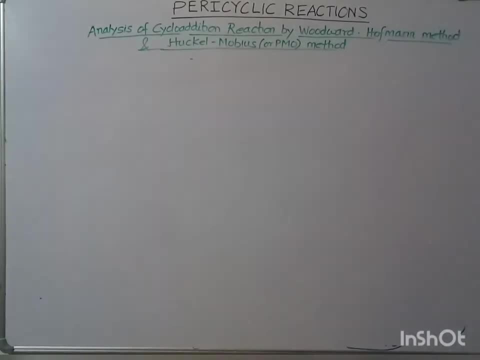 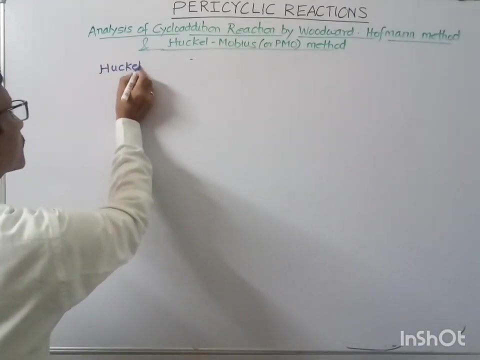 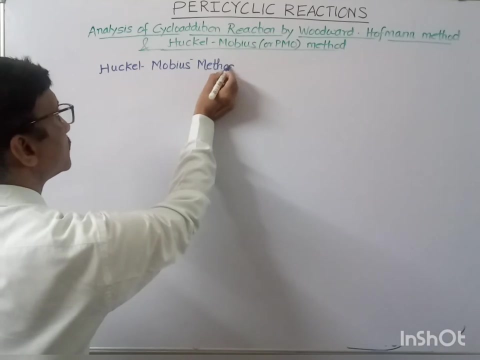 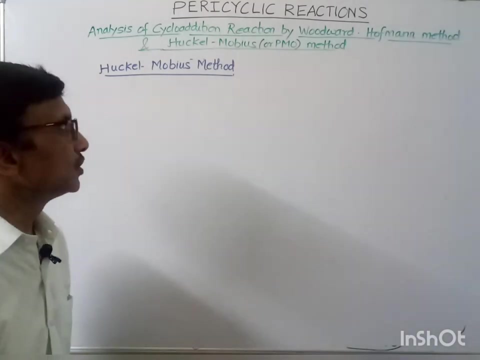 So, according to this Huckel-Mobius method. so what this called Huckel-Mobius method tells? it tells whether the load is present in a system of very tightשר favorable. 매bre, diese Huckel-Mobius method tells: it tells whether the load is present in a system of very tightשר favorable. 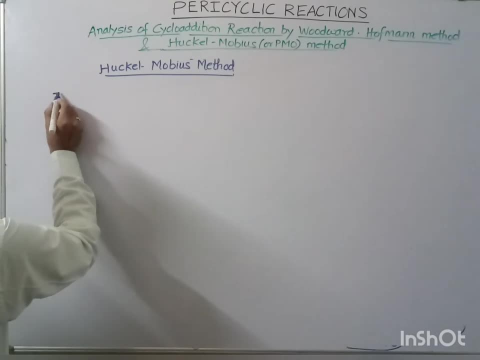 not suppose if, if there is no node. according to this view, if no node is present, in that case the system is Huckel system. the system is said to be Huckel system or Huckel array system. we can say so in this Huckel system. system is Huckel system. and suppose if 4n plus 2 electron is present, a 4n plus 2? 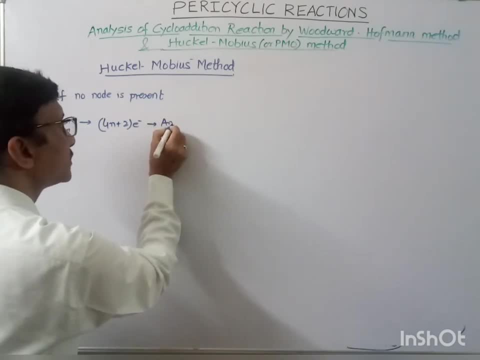 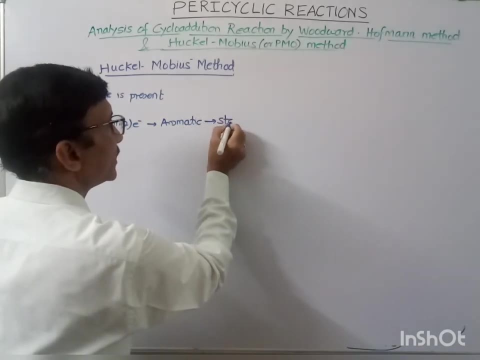 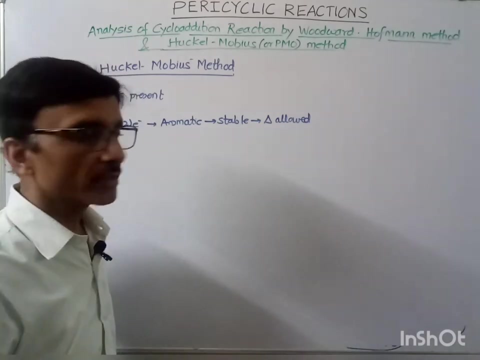 electron is present, then system is aromatic. aromatic means no doubt the aromatic systems are stable. and they are stable only under the thermal condition. this is thermally allowed. okay, now suppose in Huckel system if 4n electron is present, then the system is aromatic. or if 4n plus 2 electron is. 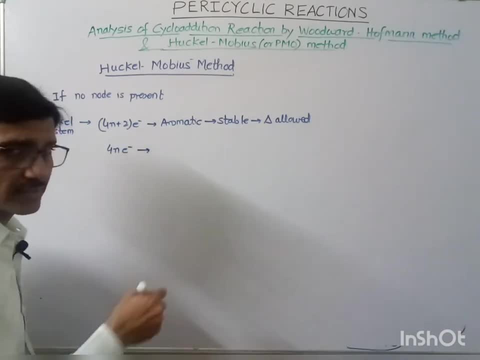 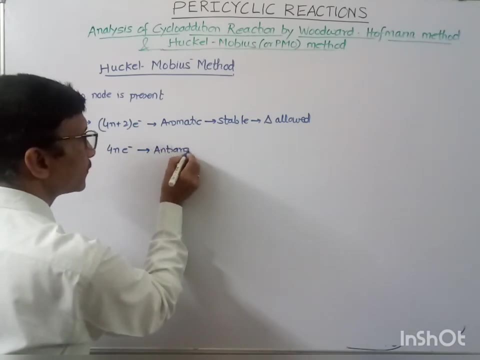 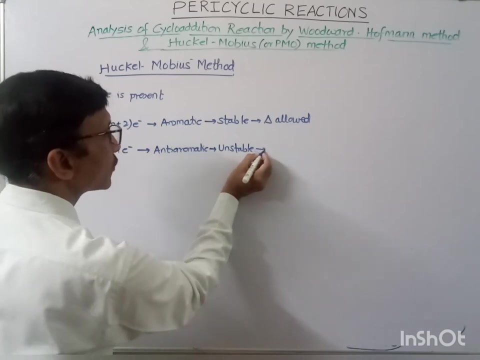 are present. We have already read the Hercule rule and if 4n electrons are present, that is said to be anti-aromatic. If it is anti-aromatic means system is unstable. When it is unstable when one of the electrons go into the excited state that is the photochemical allowed In. 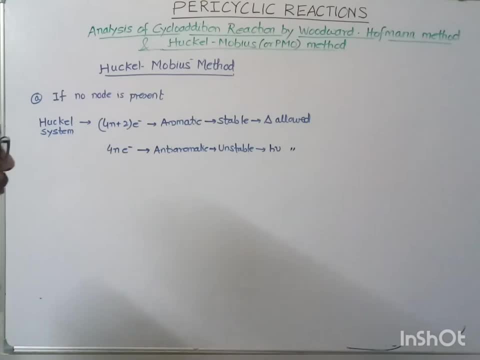 that case it means this is photochemical allowed. So this is the case when no node is present And such system is called as the Hercule system. Suppose if node is present, then such system is called as the Mobius system For Mobius array, Mobius system. Now, in this case, suppose if 4n. 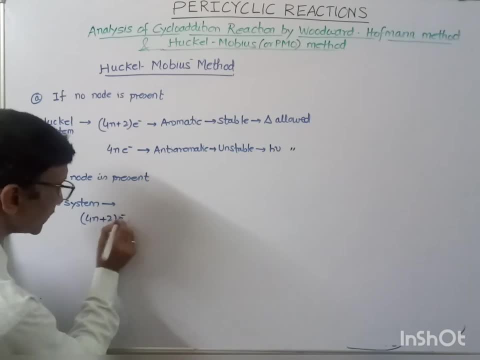 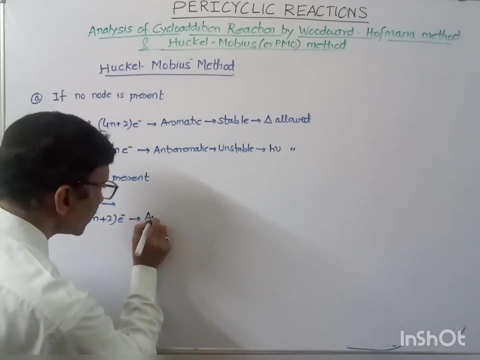 electron, 4n plus 2 electrons are present in the system, Then such system is called as the Hercule system In Mobius system. suppose 4n plus 2 electrons are present, then such system is anti-aromatic. It is just opposite to this one. It is said to be anti-aromatic. Anti-aromatic means: 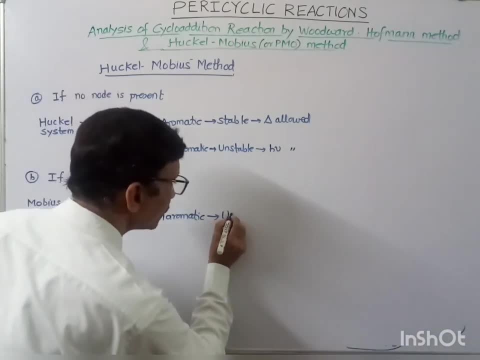 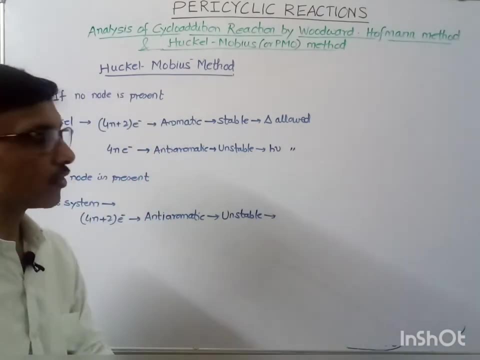 it is always unstable. Anti-aromatic system are unstable, we know, And when it would be an unstable where one of the electron will get excited from its ground state to the excited state and it get excited only in photochemical allowed. So this is the Hercule system In Mobius. 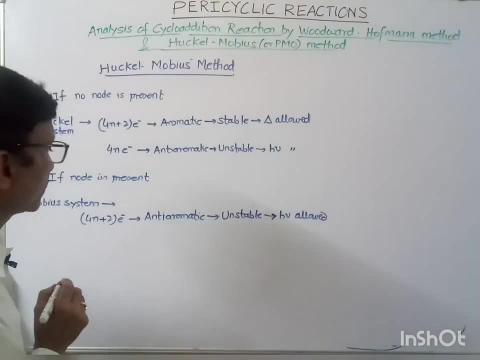 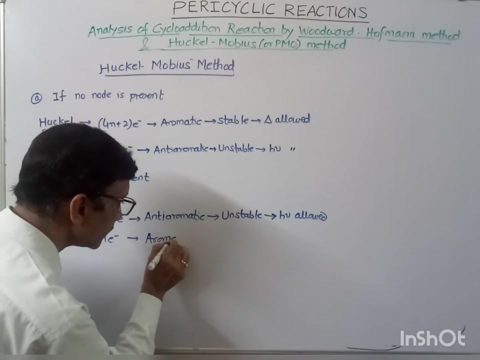 system it goes from the ground state to the excited state And for 4n electron such system if node is present. If node is present, that is Mobius system, and in 4n electrons are present, then it is aromatic and aromatic system. and it is aromatic means stable, Stable means the electrons are 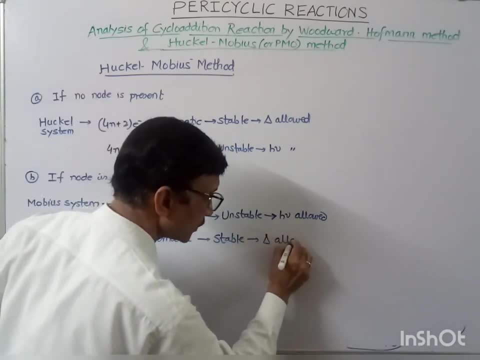 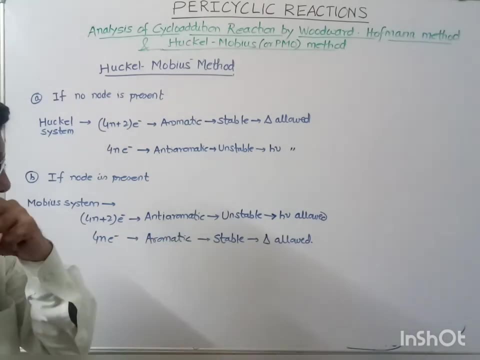 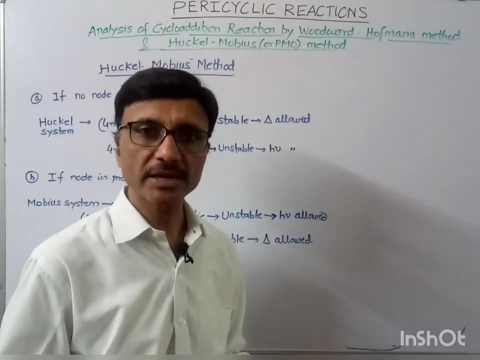 present in the ground state that is thermally allowed. Thermal, So this is the Hercule system. So this is about the rule. So this is the Appel-Mobius rule Now, so we may check for the cycloaddition reaction, the selection rule. as I have seen, We have to check the selection rule for the cycloaddition. 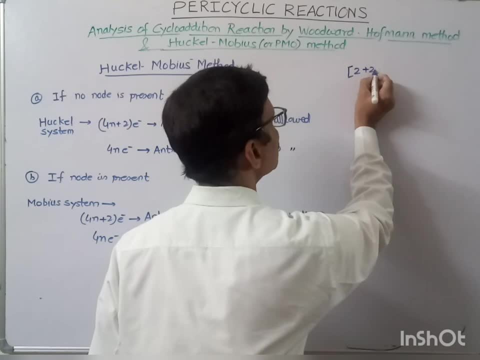 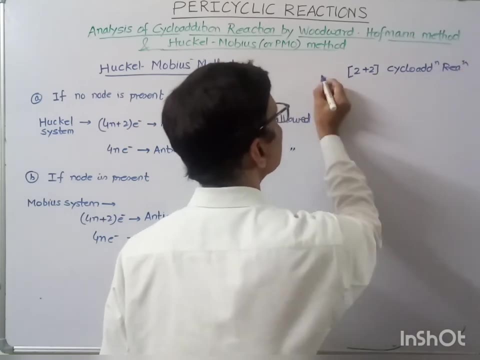 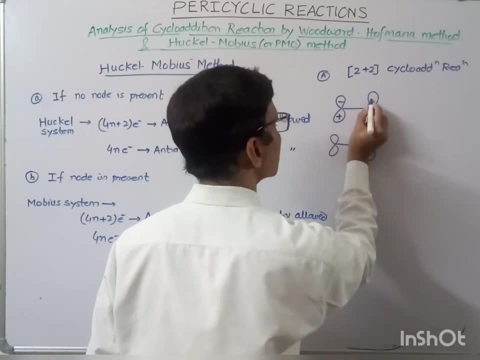 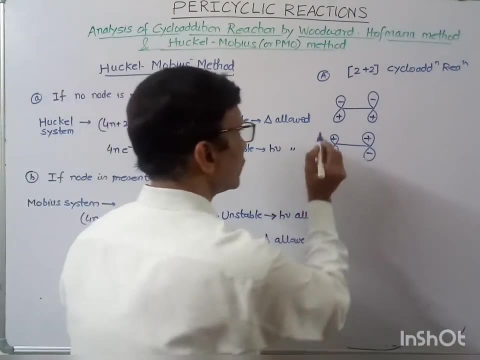 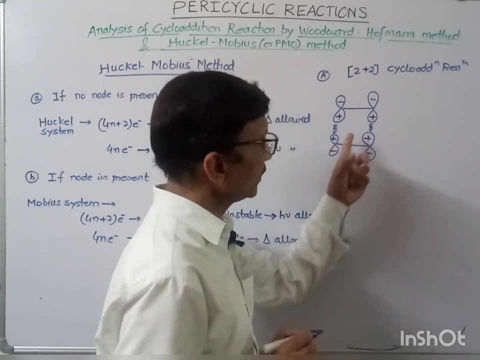 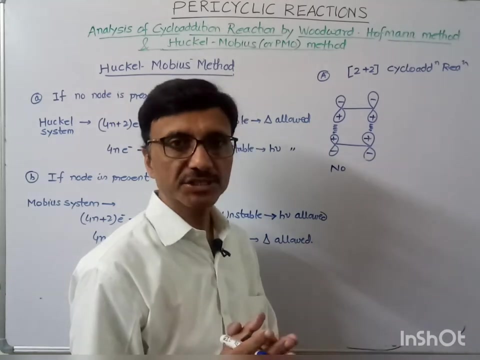 so plus plus, minus, minus, plus, like this we should see. take the sign like this: now this one, it may interact in this way. okay, so here you will find no node, because plus plus interaction gives no node. plus minus interaction gives node, so no node is present over here. if there is no node, it means the interaction it. 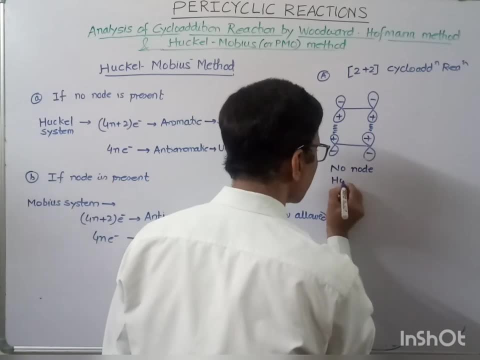 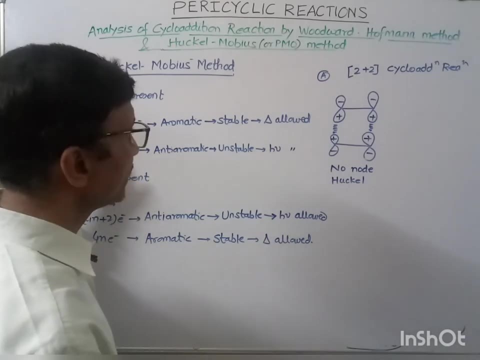 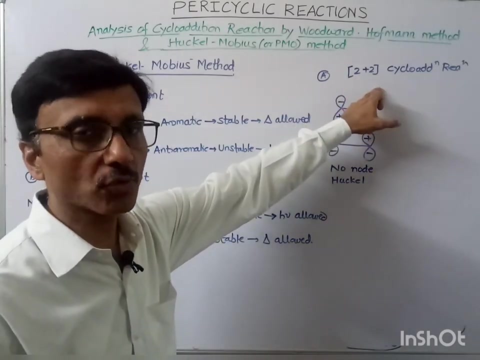 means. it means this is a Huckel system. this is Huckel system. if no node is present, it is Huckel system. and now in Huckel system, how many electrons are present over here? how many electrons are? this is two electrons. this is overall. this is four electron system. it is four electrons are present. it means this is: 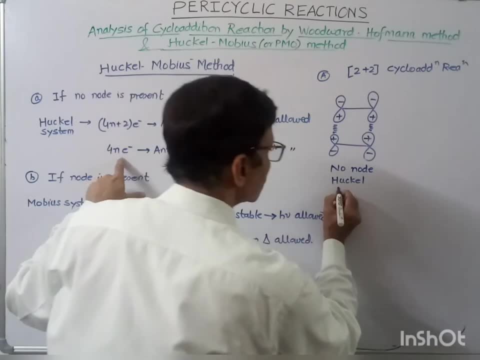 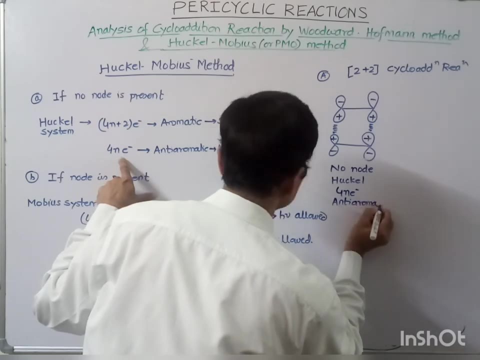 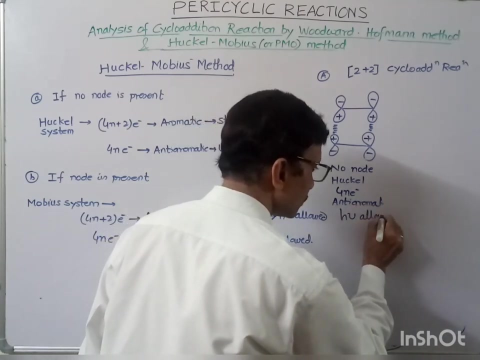 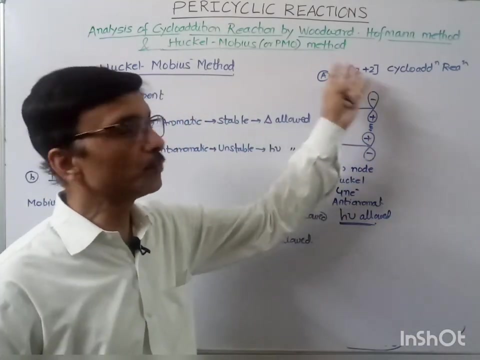 for an electron system. if it is for an electron system for an electron means this is anti-aromatic, this is anti-aromatic. anti-aromatic means this is unstable. unstable means this is photochemically allowed. this is photochemically. so we have seen the for 2 plus 2. 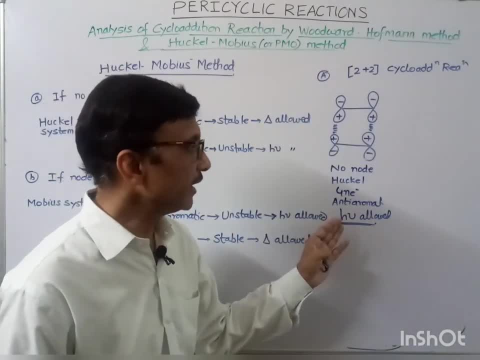 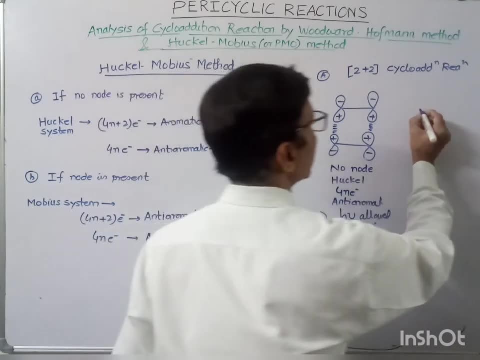 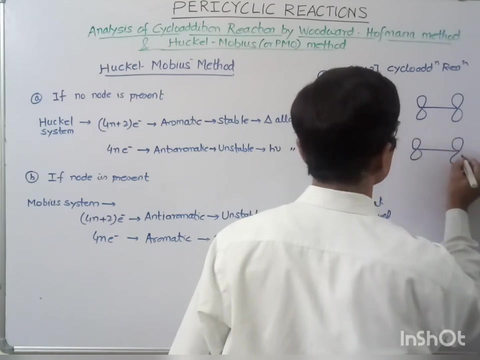 cycloaddition reaction for 2 plus 2, cycloaddition reaction under photochemical conditions. suprafacial, suprafacial infraction takes place. now suppose, if you take the suprafacial and intrafacial interaction, suppose the interaction is like this and suppose during the interaction you find one of 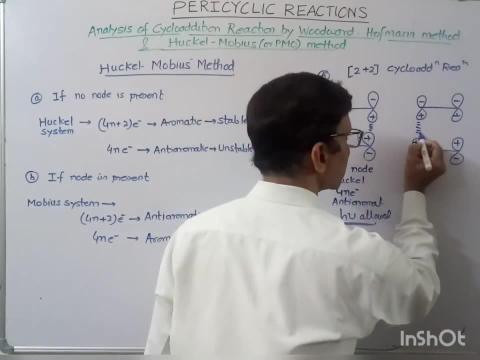 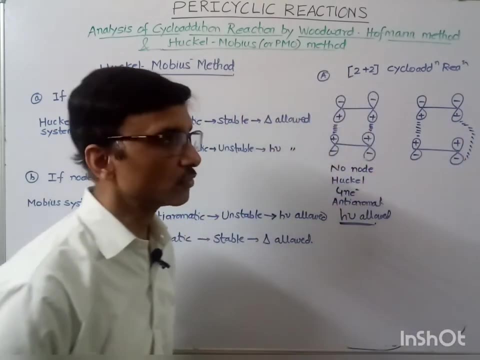 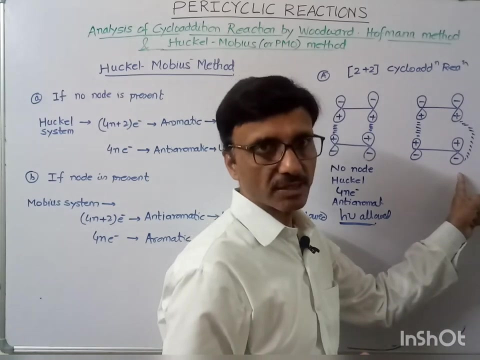 the node. so how suppose this is like this interacting in this way and this interacting? this is interacting with this opposite log, that is minus log. so you can see this plus is now combining with minus, so that in this case you will find one node, so node is present over. 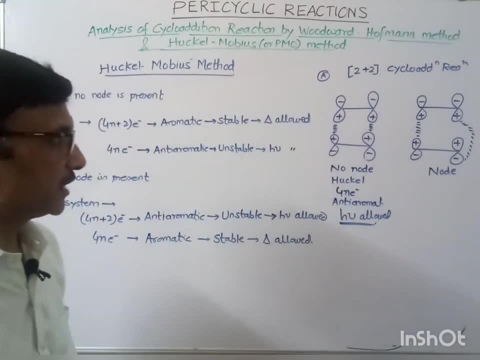 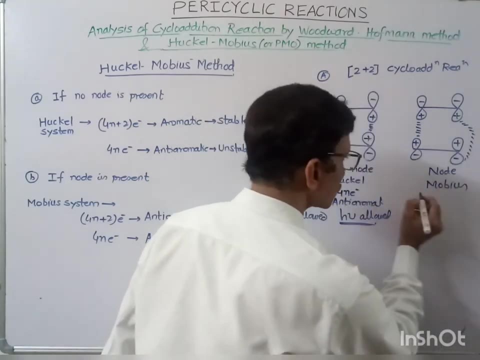 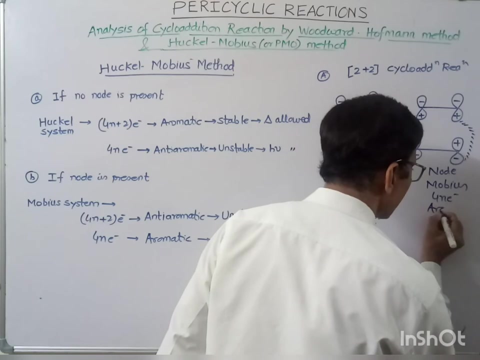 here. so if node is present, then system is mobius, one system is mobius and no doubt this is also 4n electron system and mobius system having 4n electron. this is aromatic, and aromatic means this is thermally allowed. so same rule that I. 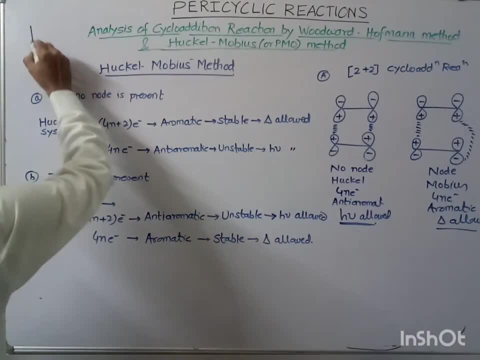 told you. so rule was: what was the rule? rule was: this was the rule for 4n electron thermally allowed, photochemically allowed, thermally allowed when it was thermally allowed when suprafacial, entrafacial or entrafacial suprafacial photochemically allow, suprafacial. but this I have proved so under. 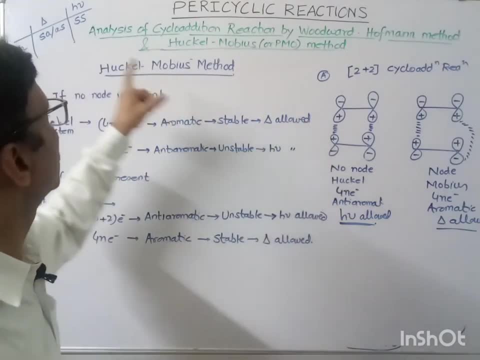 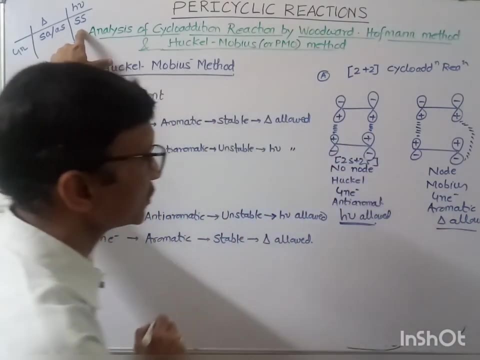 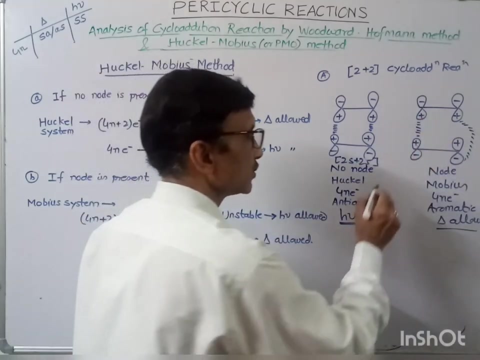 photochemical condition. what kind of interaction for suprafacial suprafacial. so this interaction is 2s plus 2s, that is suprafacial suprafacial interaction under thermal condition. what we have proved it is suprafacial entrafacial interaction will takes place. that is, this is 2s and this. 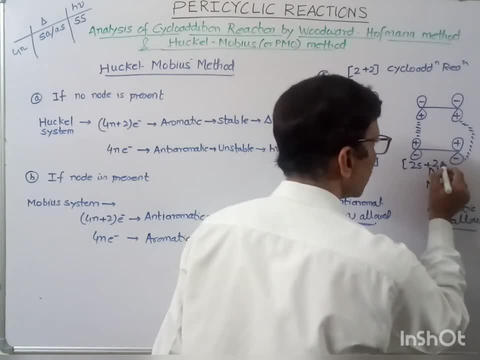 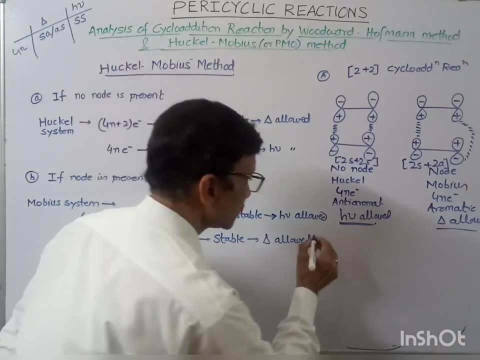 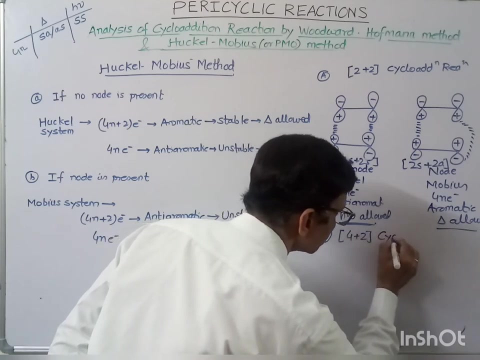 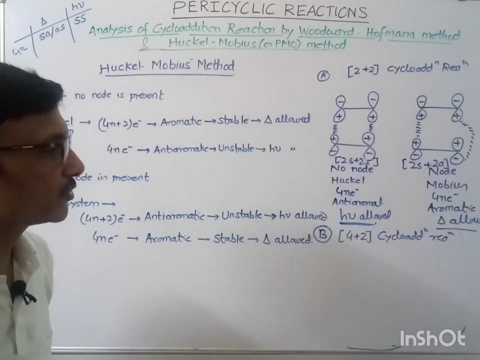 is interacting, the opposite lobes are interacting. that fight is 2s. okay. so this is for 2 plus 2 cycle addition reaction. in a same way, we may prove for 4 plus 2 cycle addition reaction. now 4 plus 2 cycle addition reaction, that is butadiene and ethene system. so 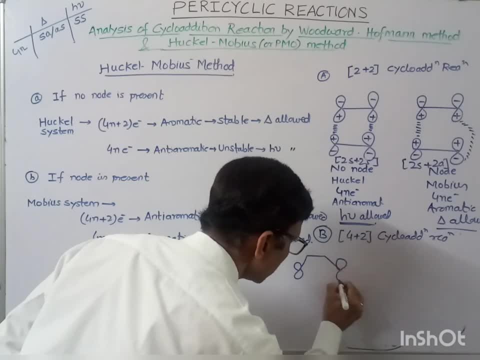 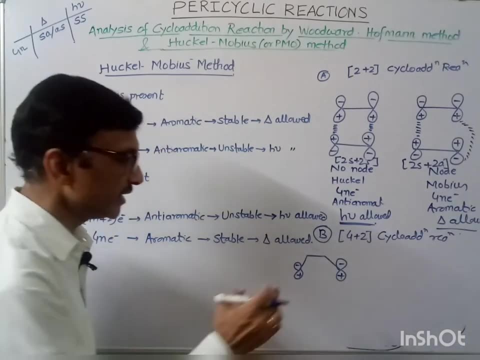 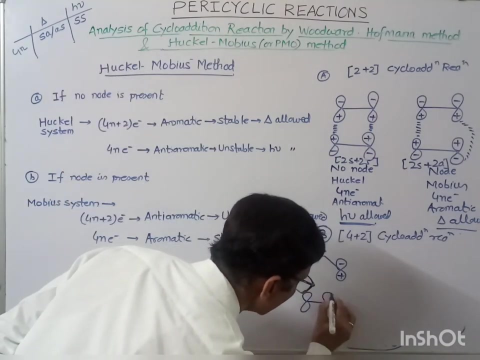 let us see, suppose this is butadiene, positive, negative. we are only concerned with the end orbitals, we are not concerned with the middle orbitals, because only end orbitals takes part in a this reaction here. so here, this is your ethene system, here also, plus plus, minus. these are the end orbital of the 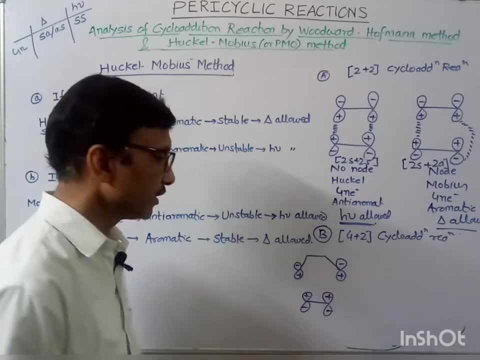 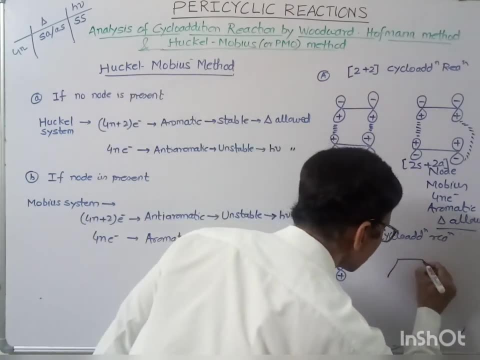 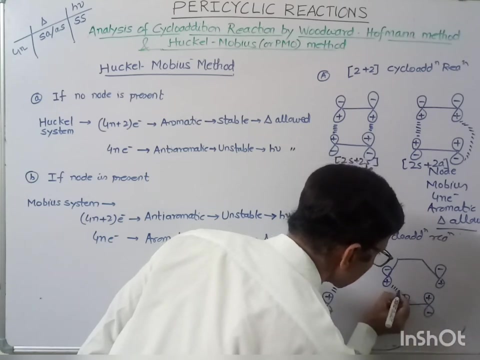 this is dynophile, this is dyn, this is dynophile. now it may interact. either this is one of the interaction or this may interact in a superficial and traficial manner. second type of interaction. so like this, this may interact in this way, so this will interact like this. so 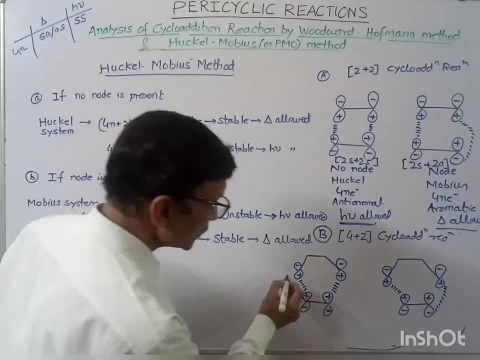 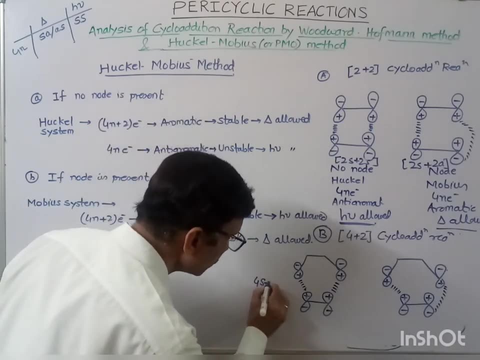 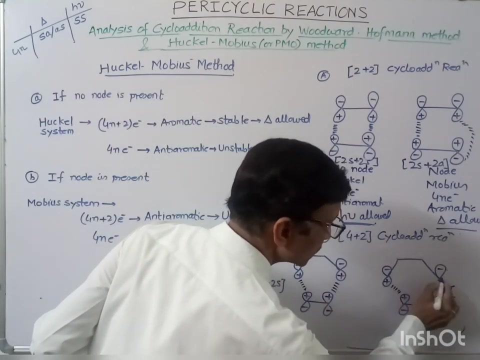 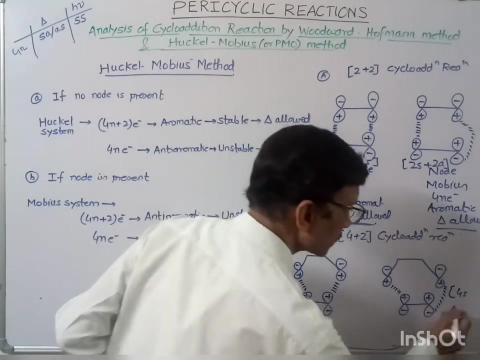 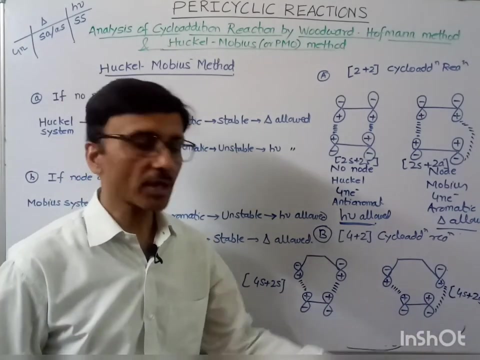 what kind of interaction this is, what kind of interaction you can write: this is 4s and this is 2s, even as we have shown wrongly. so this same side slope, same side lobe. so that's where it is: 4s plus 2s interaction. 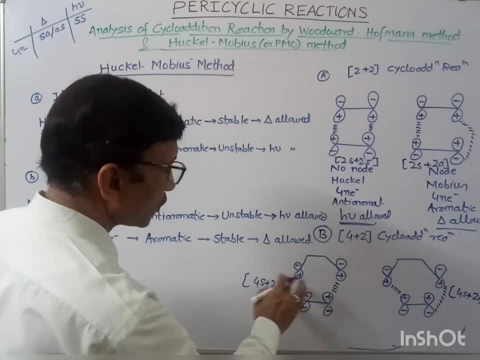 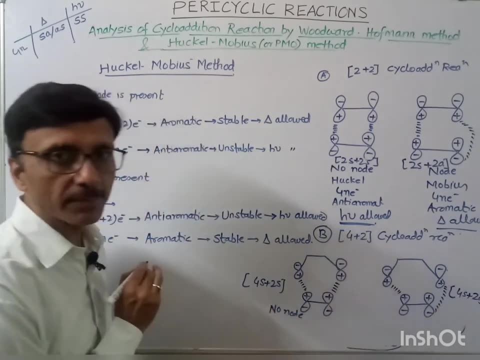 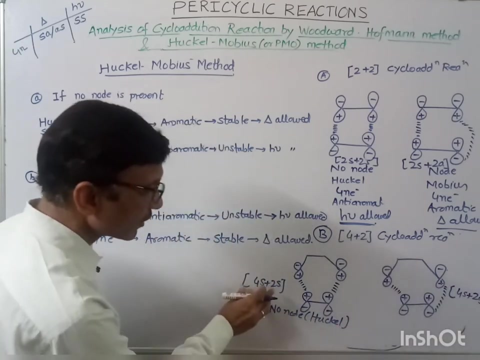 what about this? what kind of interaction this is. you can write: this is 4s, for This is: this contains no node. No node. If no node, it means what type of system this is. This is Huckel system, This is the Huckel system, And Huckel system having the how many electrons are? 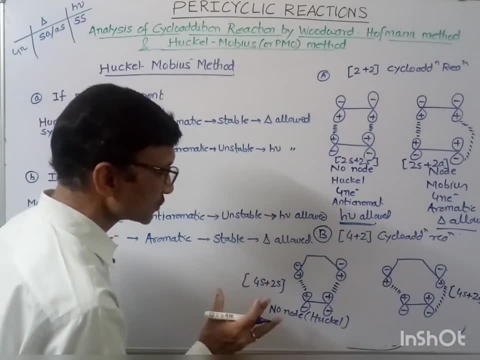 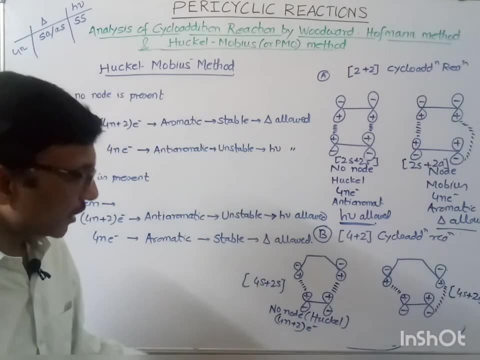 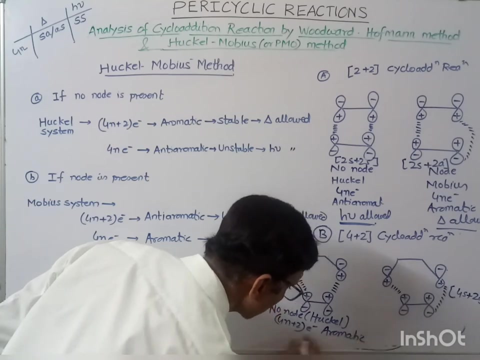 involved in this system. Six electrons are involved. So if six electrons are involved it means it is four n plus two electron system And Huckel system. Huckel system having four n plus two electron system, they are aromatic. Aromatic means stable, Stable means they are. 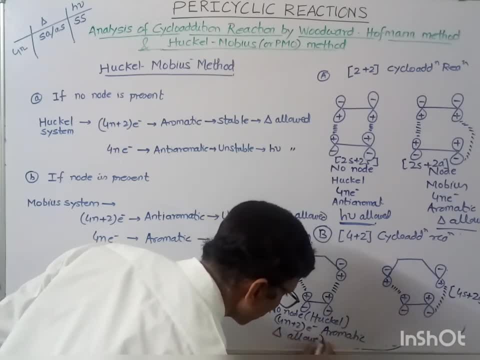 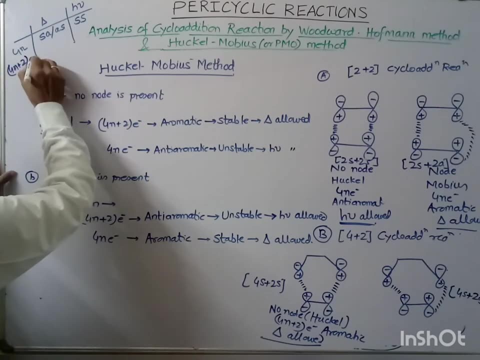 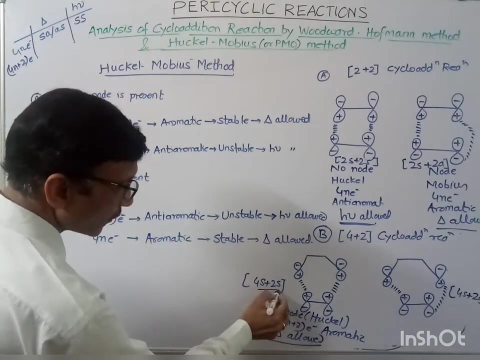 thermally allowed. They are thermally allowed. So what same thing I have written in four n plus two electron system, four n plus two electron systems under thermal condition. what kind of interaction Under thermal condition, suprafacial, suprafacial interaction takes place. Okay, Now 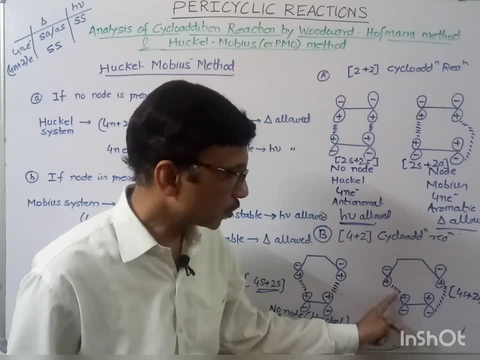 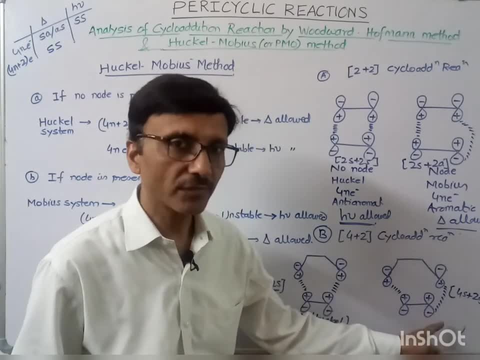 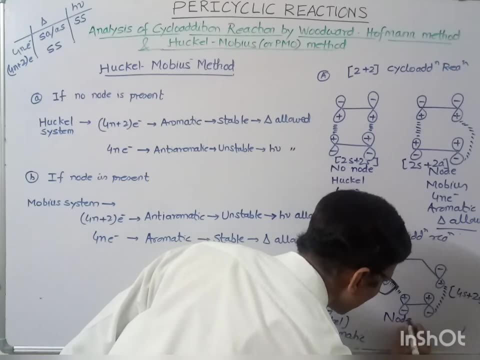 Here no node, But here one of the node is there. when suprafacial, inter-phreceial interaction, During suprafacial and inter-phaceal interaction, node is present. And if node is present it means it is Mobius system. And If it is Mobius system, if it is,